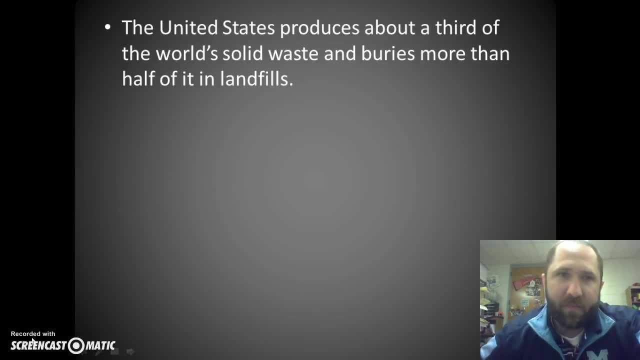 corrosive, flammable or toxic. Here in the United States we produce about a third of the world's solid waste and we bury more than half of that into landfills- About 98.5 of that. percent of that is going to be industrial waste and 98.5 percent of that is going to be commercial waste. So 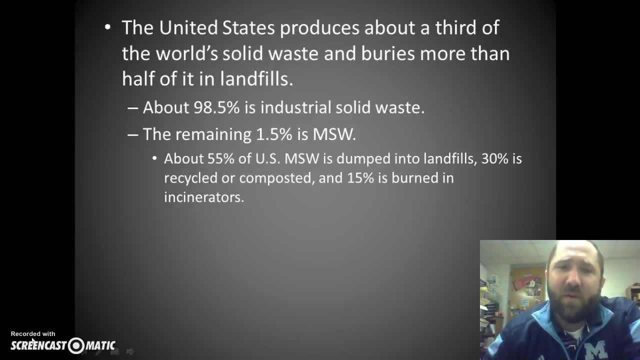 we're going to be using this to produce more of that, And that's where we're going to start. in the United States, We're going to take a look at the quality of our waste, and we'll begin by taking a little solid waste, while the remaining one and a half percent is our municipal solid. 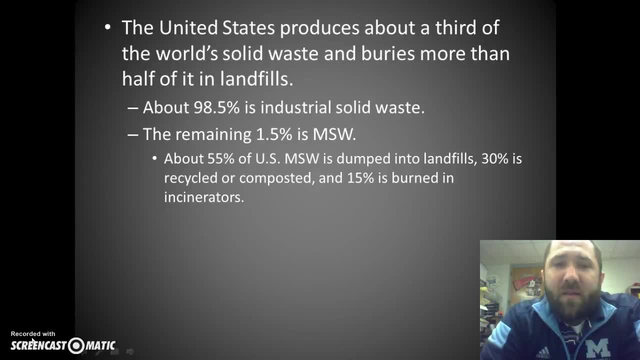 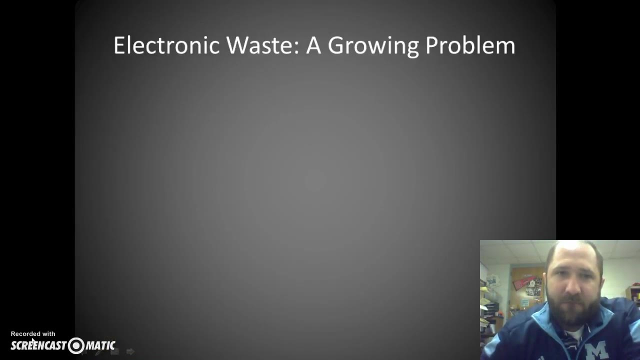 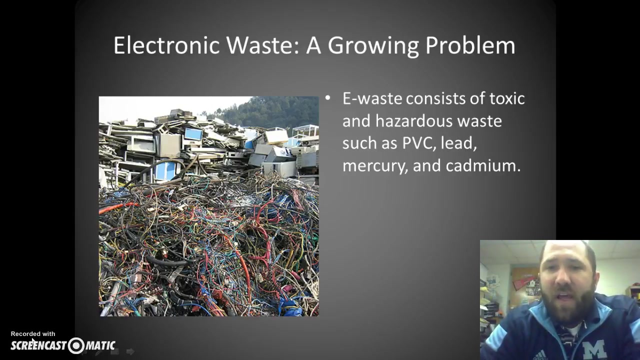 waste. here in the United States about 55% of our municipal solid waste is dumped into landfills. we recycle or compost. roughly 30% of our waste in about 15% is burned in incinerators. any of our electronic waste things coming from our computers, things like PVC, lead, mercury, cadmium- that is considered. 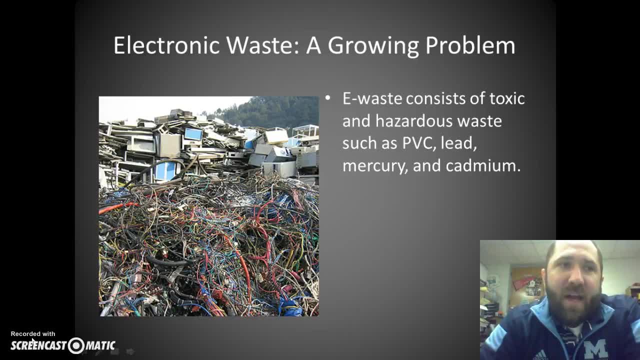 e-waste and with our ever-growing society and becoming more technologically advanced, that is becoming a bigger problem because of the fact that we were producing more and more of this e-waste again, the us being the most wasteful. we produce more than half, or about half of the world's. 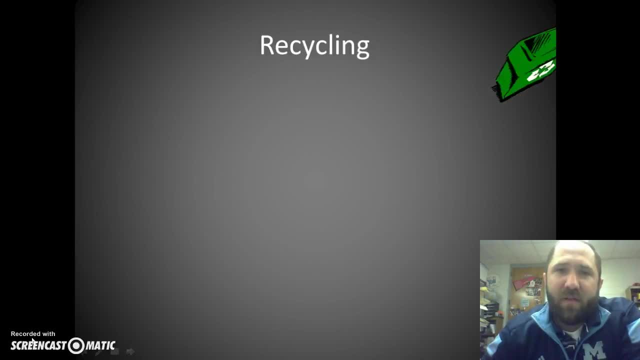 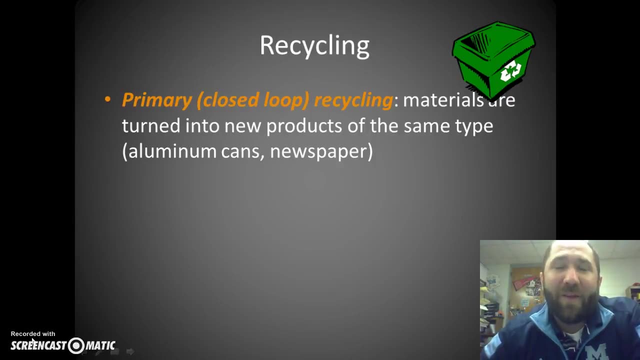 e-waste, but we're only recycling about 10% of it. when it comes to recycling the two different types- primary recycling, which is a closed group group- excuse me, closed loop recycling- and that means that the materials are just turned into new products of the same thing. aluminum cans get recycled to become aluminum. 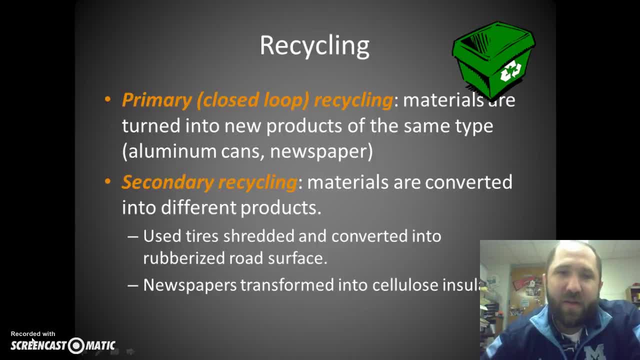 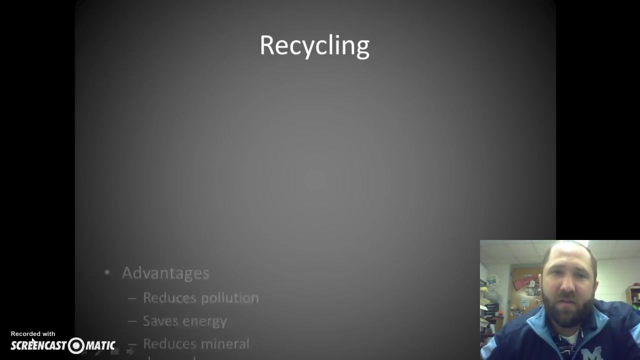 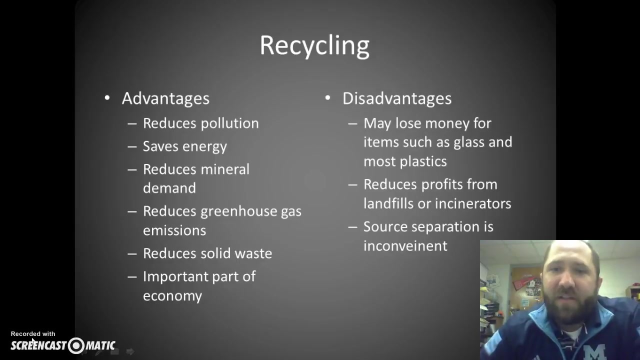 cans newspaper gets recycled to become newspaper. secondary recycling is when we take materials and we convert them into different products. we use tire shreds and we convert them into rubberized road surface or the rubber mold. the plastic, then, is what is being recycled itself. so some of it isn't not. 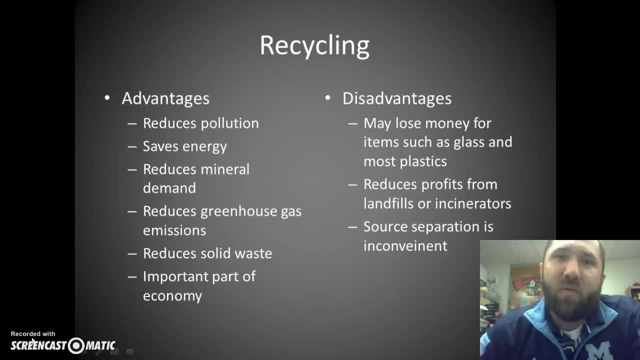 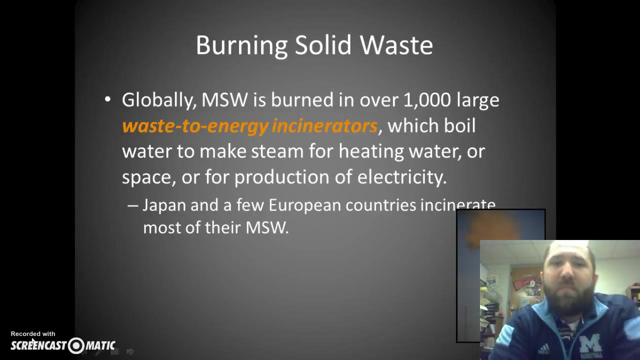 even being transferred into another plastic bottle or another material. it also reduces our profits from landfills or incinerators as well. as it's a sort, it's a separation is extremely inconvenient when we burn solid waste. globally over 1,000 large waste to energy. 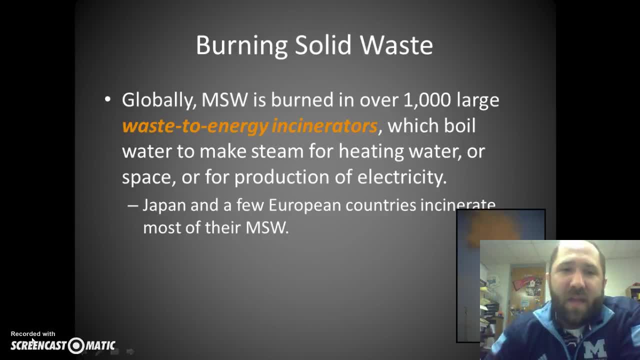 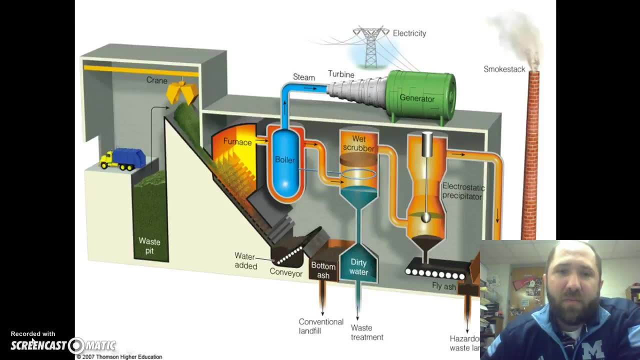 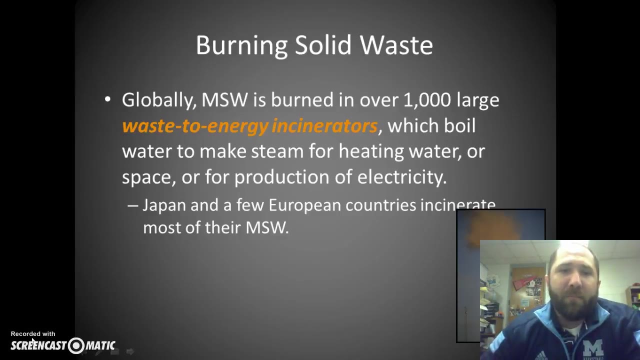 incinerators are being used and what happens in them is they boil water, that the steam produced by the boiling water is going to then turn a turbine which is then going to produce electricity in our generator. Japan and a few European countries use in incinerators for most of their municipal waste as well as. 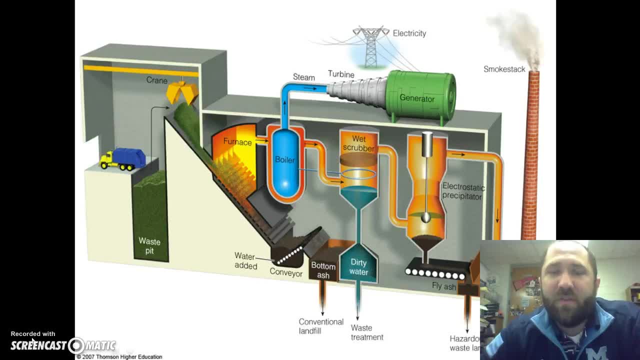 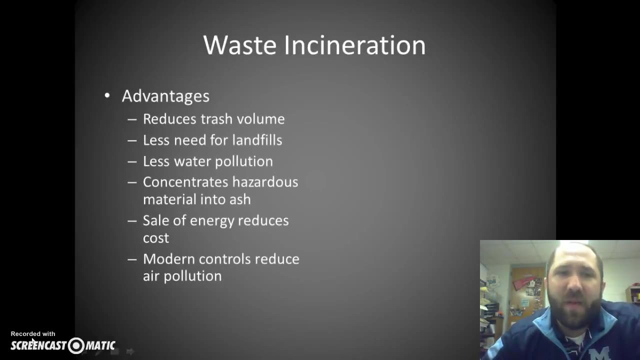 Sweden right now is currently paying other countries to bring in their wastes because Sweden is using the incinerators to create the majority of the electricity for their country. advantages to waste incineration: it's removing the large volumes of trash that we have created, as well as it creates less need for landfills themselves we don't have as 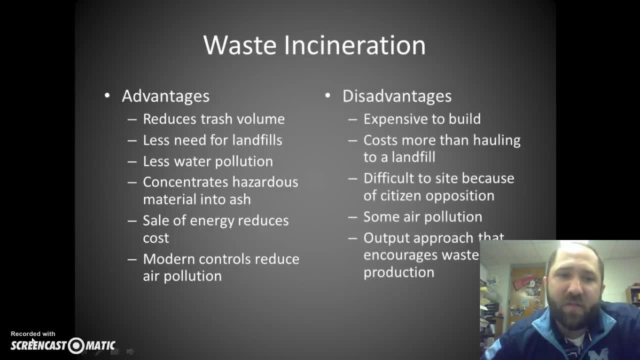 much water pollution because the trash is not just sitting there as well as the sale of energy, reduces our energy costs, disadvantages they're very expensive to build. they cost more than hauling the trash to a landfill as well as it does create some air pollution and its output approach that encourages the waste. 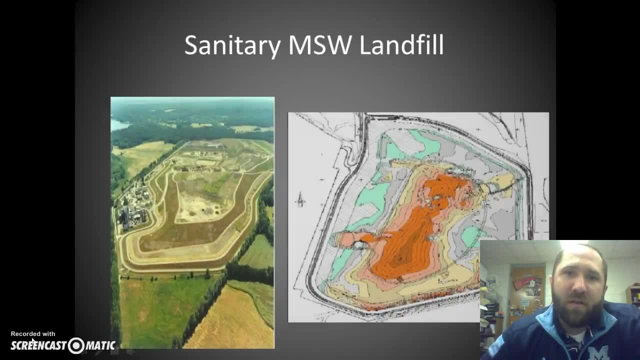 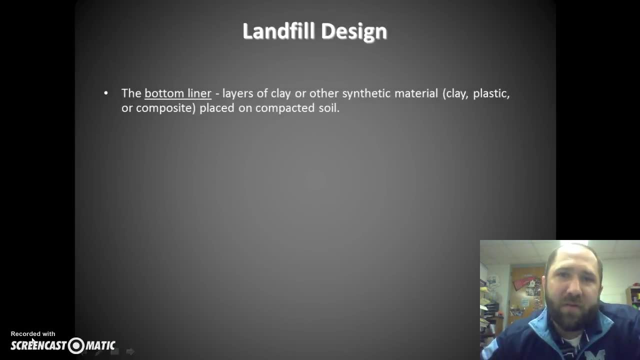 production. here's a couple images of sanitary landfills. how the landfills are designed is that a bottom layer of clay or some other synthetic material- plastic or composite- is placed on compacted soil. so we need some sort of bottom impermeable layer so that way nothing is going to drain into our groundwater. the 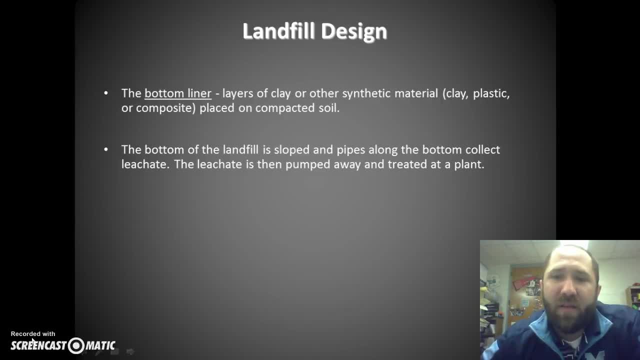 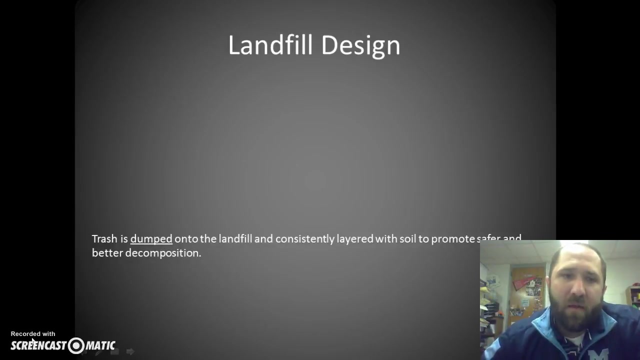 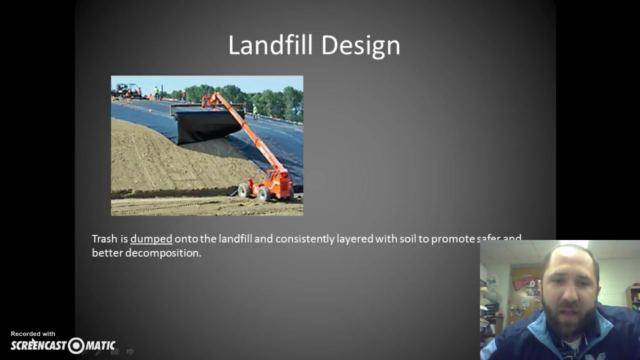 bottom then of the landfill is sloped and pipes along the bottom of that slope are going to collect leachate. anything that's going to leak through the landfill gets collected and pumped away and taken to a treatment plant to be cleaned. after that we dump our trash in. once we dump our trash in and get a good layer. 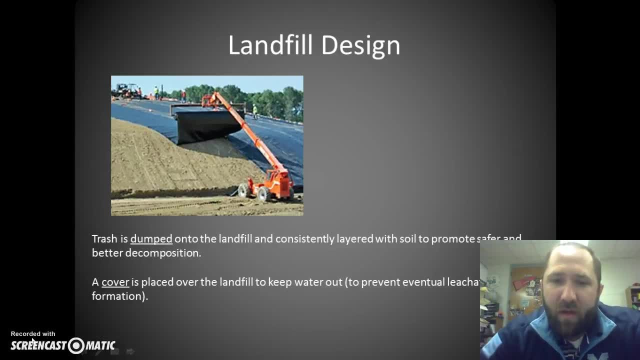 we then cover it with a liner, and that liner is to help prevent the eventual leachate from forming, because it's not going to allow water to easily penetrate into the garbage itself. between or after- excuse me, we dump the garbage, we then put a layer of soil on top of it and then 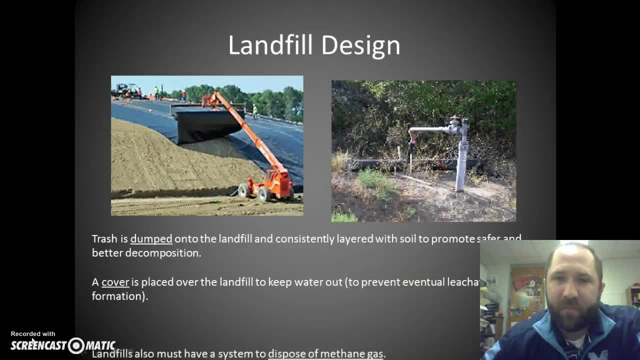 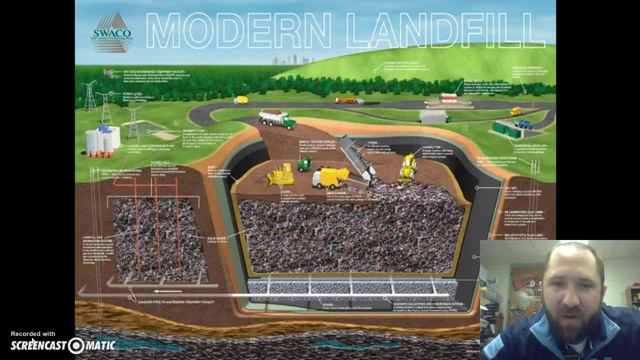 we put our liner down, you can see the picture there. you can see the pipes at the very bottom. the one thing that we do have to monitor is the methane being produced from the decomposition of all of our garbage, and so we have. we have pipes that come out of the ground and that is burning off the methane gas if 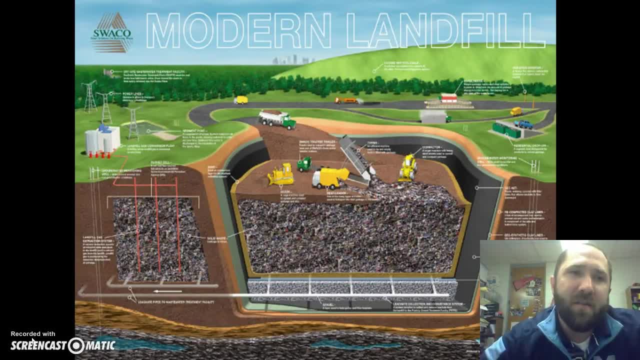 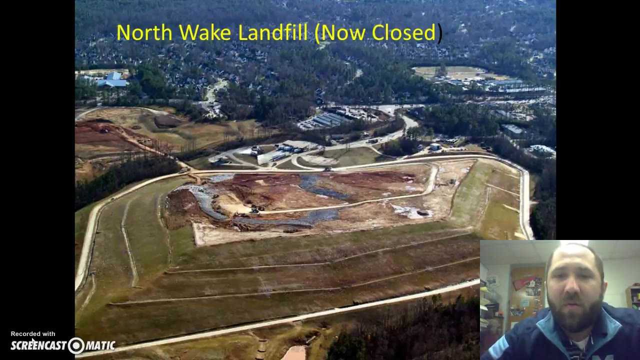 you drive by a landfill and you see a lot of the garbage and you see the constant flame coming out of a pipe in the area. that is because that methane is is being burned. the North Wake landfill, which is the landfill off of Durant Road, is now closed. there's a picture there what we, where we now ship our trash, is. 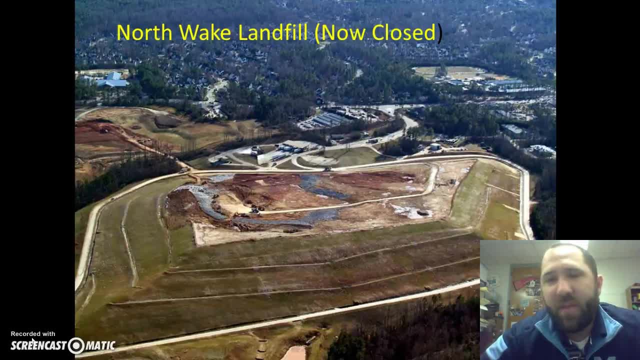 to the South Wake landfill and that is near Holly Springs, and this is another example of environmental justice. The reason that it is an example of environmental justice is because it is built in a in or around predominantly black neighborhoods, and it's something that, even though they fought the, the county still decided to put it there. because of the large open space. just like waste incinerators, there's also advantages and disadvantages to landfill. some of the advantages are that they're very little odor due to the bare, the soil barrier and the plastic liner put over top of them. they're built quickly, there's very low operating costs and it. 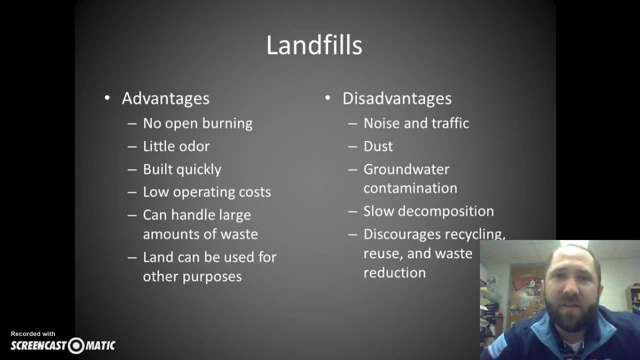 can hold large amounts of our waste. some disadvantages are all of the noise and traffic created because of the trucks moving in and out to dump the waste, large amounts of dust going on during the process of building the landfill up layer by layer, and the potential of the groundwater contamination due to the 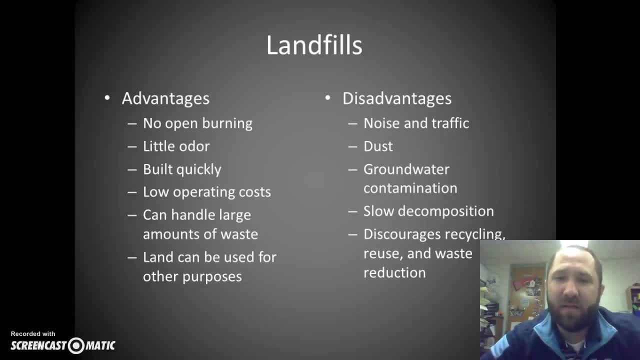 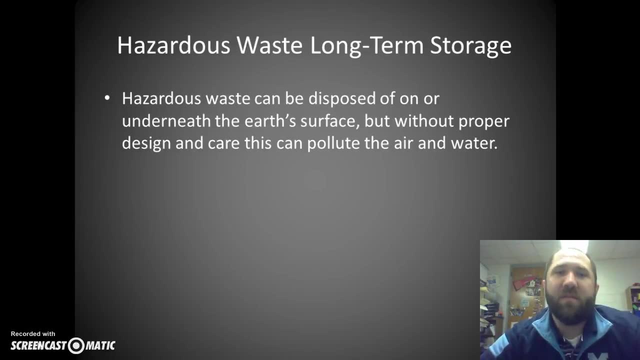 leachate not being fully collected. hazardous waste needs to be stored long term and we can dispose of this underneath Earth's surface. but without proper design and care for the hazardous waste it has dangerous effects to pollute our air and water. Deep well disposal is what we do with our liquid hazardous waste: we pump them. 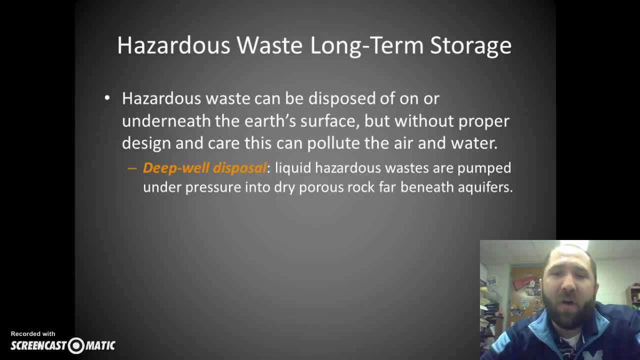 under pressure deep into a dry, porous rock far beneath our aquifers. we pump them into the porous rock far below our aquifers because we do not want gravity to take effect and allow this- the hazardous chemicals- to make their way into the aquifer surface. impoundments are when we just excavate depressions. 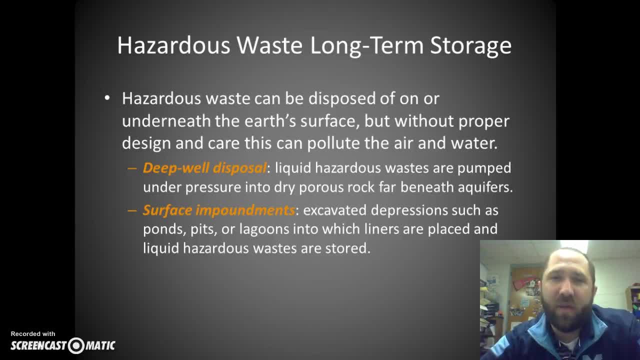 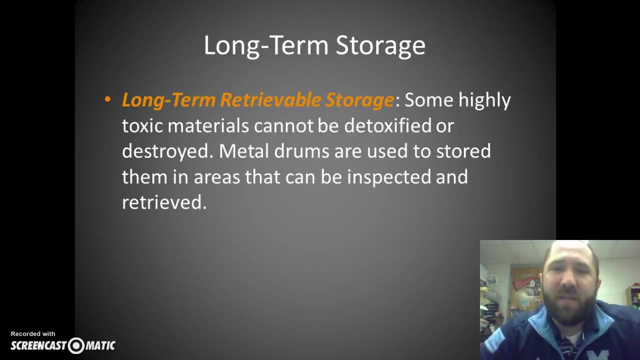 and these can be things like pits, ponds or lagoons- and we put down a impermeable liner and then we dump all of our hazardous waste on top of that liner and store it. that way, for waste that are not able to be detoxified or destroyed and things that we need to be able to retrieve, we put 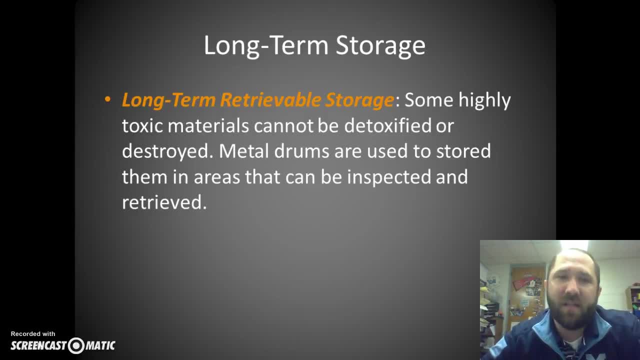 them in metal drums and we just store them in an area that we can constantly inspect them and retrieve them when necessary. secure landfills are set up a lot like a our sanitary landfills. we put the hazardous waste into drums, we bury it carefully in a designed landfill and then we place monitoring systems in. 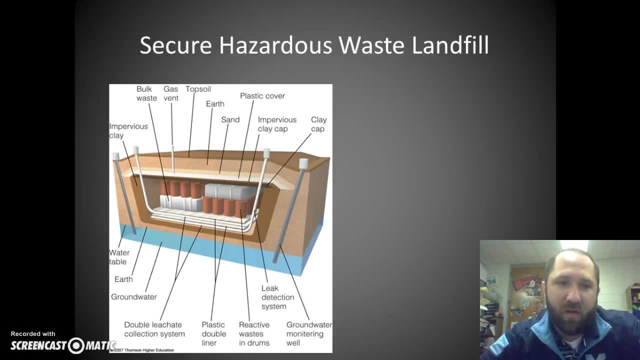 there. this image shows you what that might look like. we have in there different ground watering monitor wells on both sides of the landfill itself, as well as an impermeable clay bottom. then inside of the actual landfill we have another monitoring system detecting any leaks that may occur from the drums, and then on top of the drums we put down a clay. 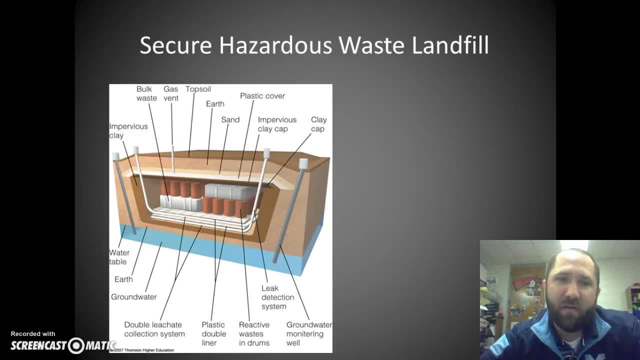 cap, a plastic liner, and then we have our sand, eventually our subsoil and topsoil on top of that, all of which to try to make sure that none of the toxins can get released into the groundwater or make its way up to Earth's surface. 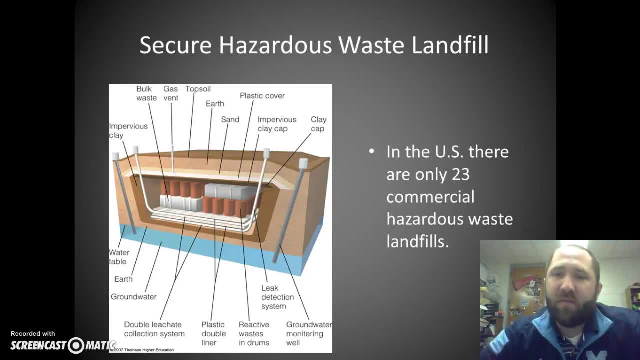 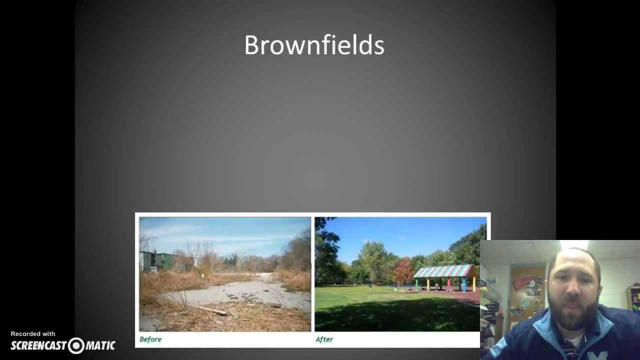 here in the United States we have a lot of landfills that are not able to be reused. in the in Las Vegas I would mention events like the boards at the brownfields home, where we had landslact at the brownfield site this same winter before the.